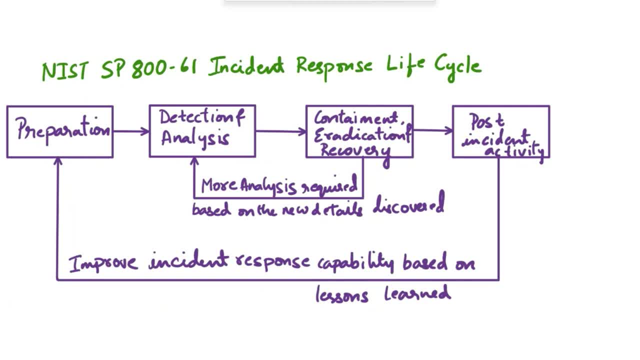 that are related to cyber security. For example, NIST SP 853 is related to security and privacy controls. NIST SP 800-171 is related to protecting controlled unclassified information in non-federal systems and organizations. NIST SP 830 talks about risk assessments. So to summarize, 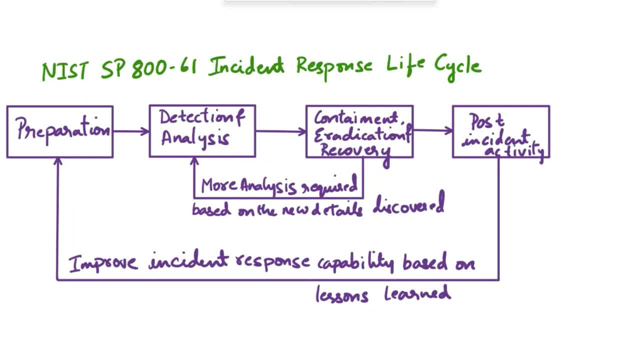 these publications provide comprehensive guidelines, standards and frameworks that organizations can use to assess risks, implement security controls, respond to incidents and establish effective cyber security programs. Today, in particular, we'll talk about 861.. 861 stands for computer security, NIST SP. 830 talks about risk assessments. So, to summarize these publications, 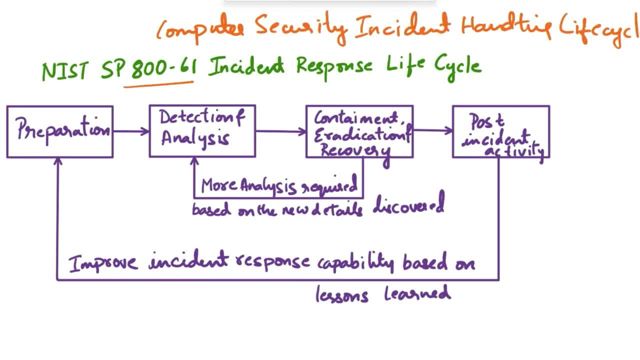 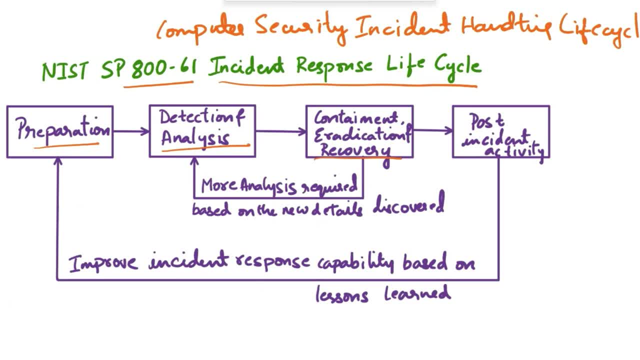 provide comprehensive guidelines. NIST SP 830 talks about risk assessments. So, to summarize, these publications provide comprehensive guidelines. So, to summarize, these publications have been presented in feel the cyber security process, Last slide. please Just a few само examples to come up. if you want to go into the details of this full analysis皆さん can go to. 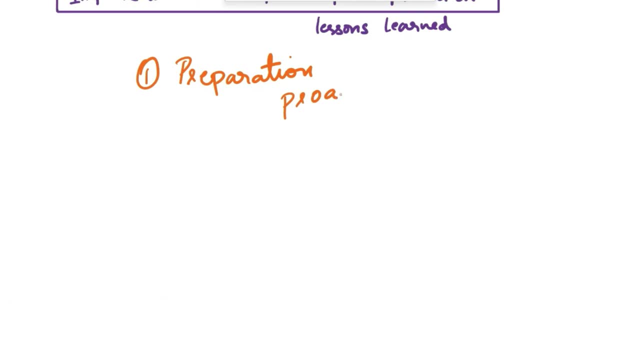 LYNACOM's website, Facebook, Twitter, 2015 blog is there. Its link is on the top right of the screen. This digital everything passing über Top priority. we upload the video After configuration ourselves. next we will work with you to figure out why our framework has been given. 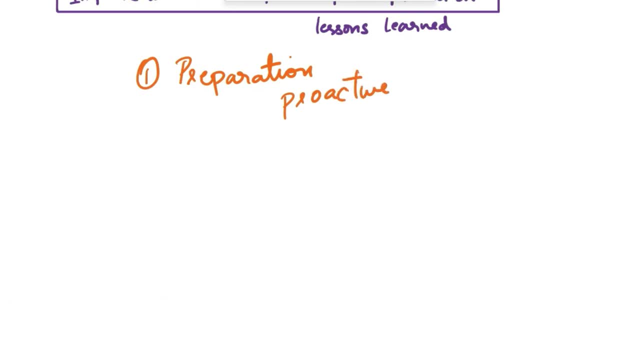 to prepare for potential security incidents. Let's discuss some of the aspects of the preparation phase. First one is incident response policy and plan. Here we develop an incident response policy that outlines the organization's commitment to incident handling and establishes the objectives, scope and authorities for incident response. And then we create an incident response. 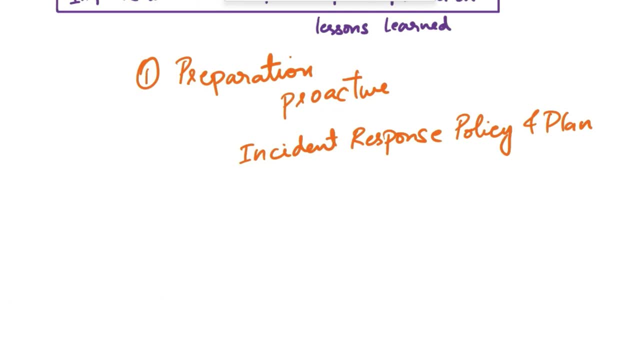 plan that provides detailed procedures and guidelines for responding to incidents. The plan should cover various types of incidents, roles and responsibilities, communication protocols, coordination with external entities, etc. The next aspect here is incident response team. Here an incident response team is formed. This team is comprised of individuals with the necessary skills. 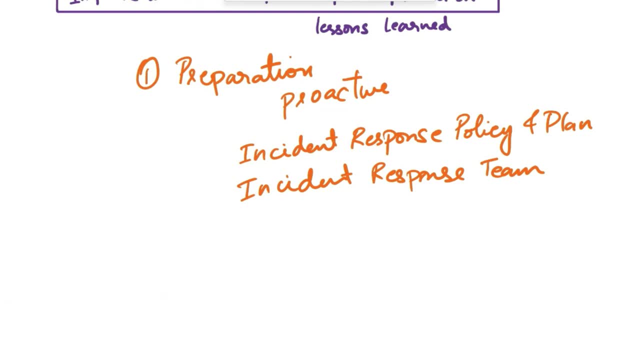 and expertise to handle security incidents. Here we define roles and responsibilities for team members, ensuring clear lines of communication and decision making during incident response. And then we have training and awareness. Here we provide training and awareness programs to educate employees, including incident response team members. 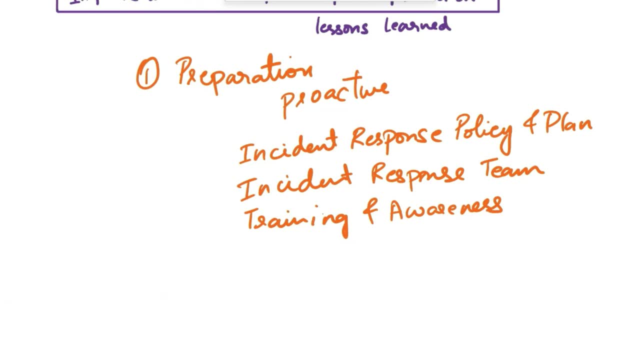 and other stakeholders about their roles and responsibilities in incident handling. We conduct regular exercises and simulations to test the effectiveness of the incident response team. The next aspect is communication and coordination. Here we try to establish communication channels and protocols for incident reporting escalation and coordination within the organization. This 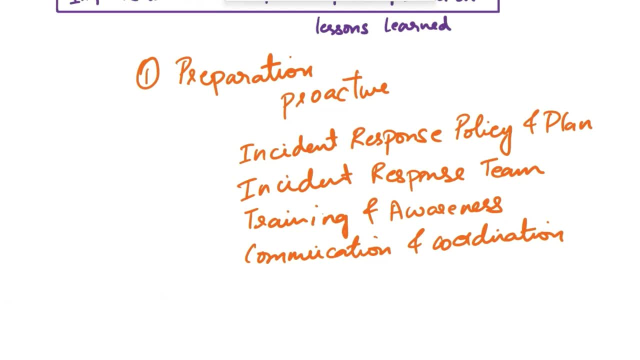 includes defining points of contact and establishing relationships with external entities such as incident response teams, law enforcement agencies and regulators. Next aspect is tools and resources. Here we identify and acquire necessary tools, software and resources to support incident detection, analysis, containment, eradication and recovery activities. This may include intrusion detection systems, log management solutions, forensic tools, incident response platforms, etc. 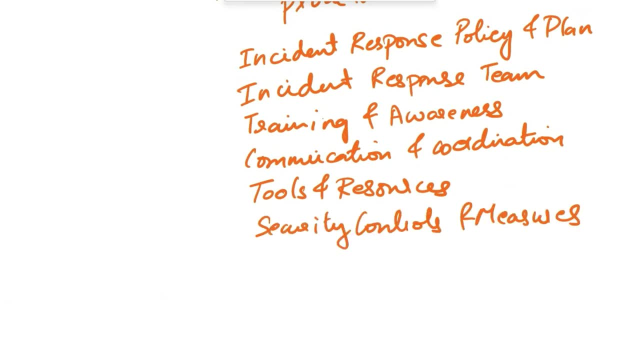 And then we have security controls and measures. Here we implement appropriate security controls and measures to prevent, detect and respond to security incidents effectively. This may include network segmentation, access controls, encryption, logging and monitoring mechanisms, incident response, specific technologies and so on. Next is documentation and reporting. 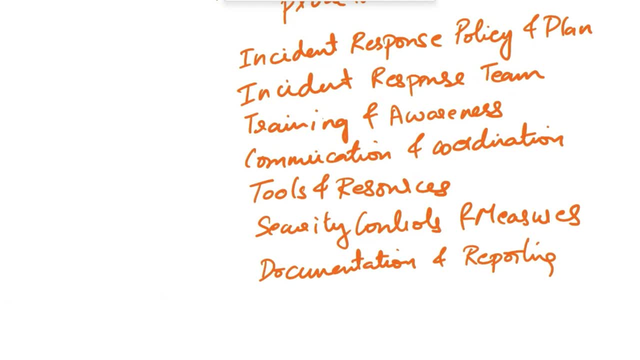 Here we establish guidelines and templates for incident documentation, including incident reports, logs and records. We also define the process for collecting, analyzing and preserving evidence during incident response activities. So, basically, the preparation phase lays the groundwork for a well-organized and coordinated incident response process By having a documented incident response policy, a well-defined incident. 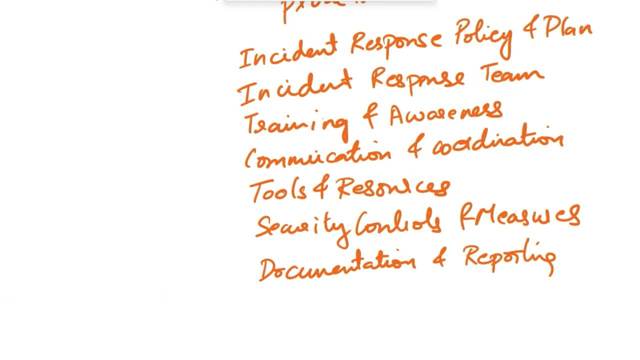 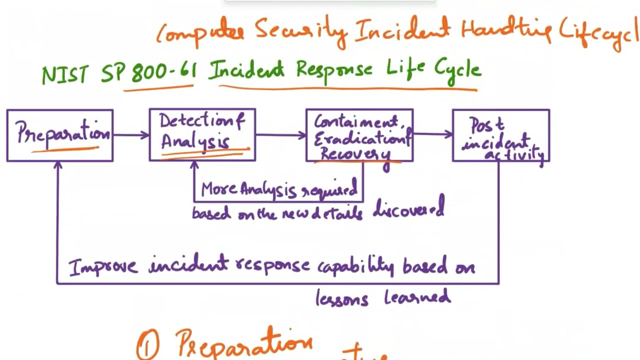 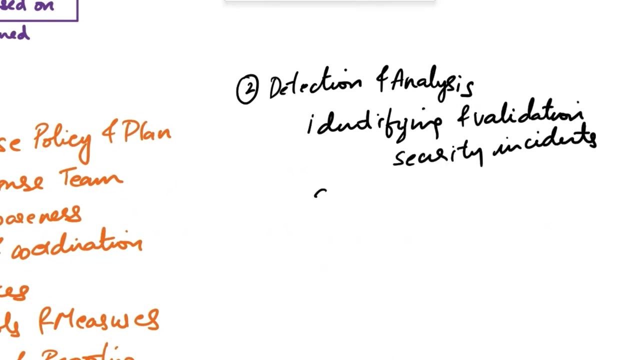 response plan, a trained incident response team and the necessary tools and resources, organization can be better prepared to handle security incidents effectively and efficiently. So now we know about the preparation phase. The next one is the detection and analysis phase. This phase focuses on identifying and validating security incidents, as well as gathering. 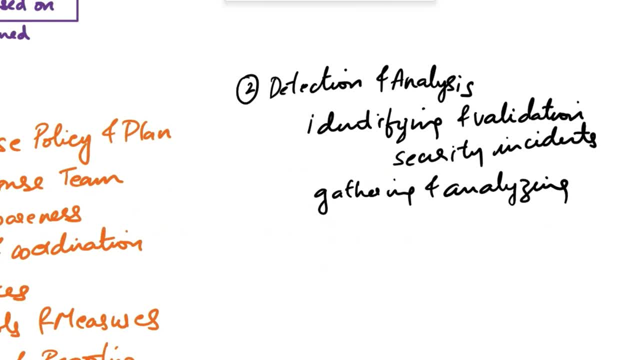 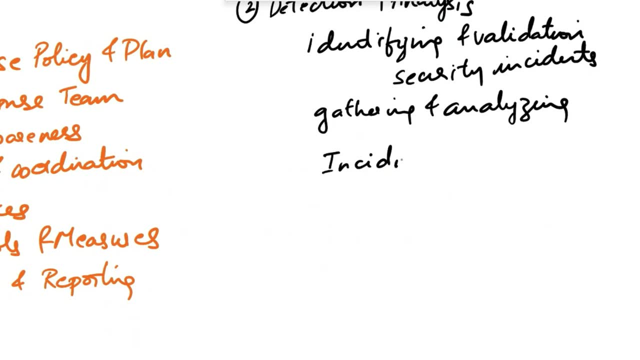 and analyzing relevant data to understand the scope and impact of the incident. Let's see some of the key aspects of this phase. The first one is incident identification. Here we monitor systems, networks and security controls. and then we identify and validate the incident. Here we monitor. 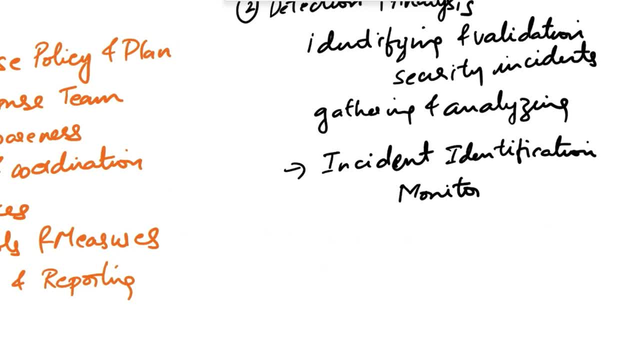 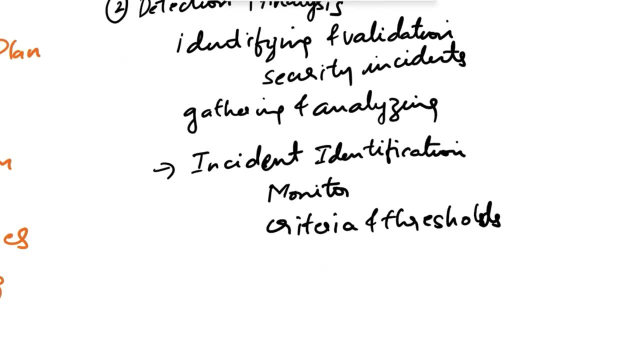 detailed burner reports, perform pullups and alerts to detect potential indicators of compromise or suspicious activities, and then establish criteria and thresholds for identifying security incidents based on predefined rules, alerts or anomalies, And then receive reports from users, automated systems or other sources that may indicate a potential security incident. 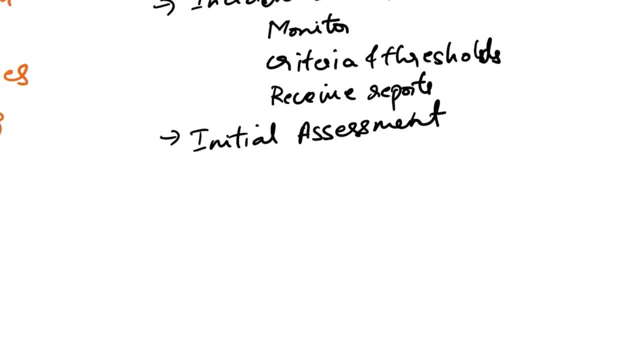 The next one is initial assessment. Here we assess the reported incident or to determine if they meet the predefined criteria for a security incident, conduct an initial triage to prioritize incidents based on severity, potential impact and criticality, and then assign incident handlers or teams to investigate and respond to each incident based on their 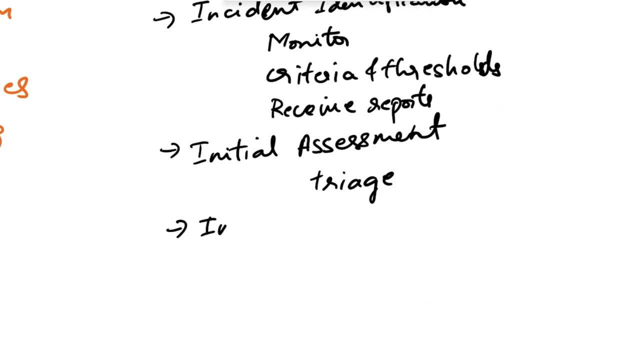 expertise and availability. And then we have incident validation. Here we validate the reported incident by gathering additional evidence, logs, system snapshots or network traffic data. We verify the accuracy and legitimacy of the reported indicators through further analysis and investigation. We also determine if the incident is a false, positive, an actual. 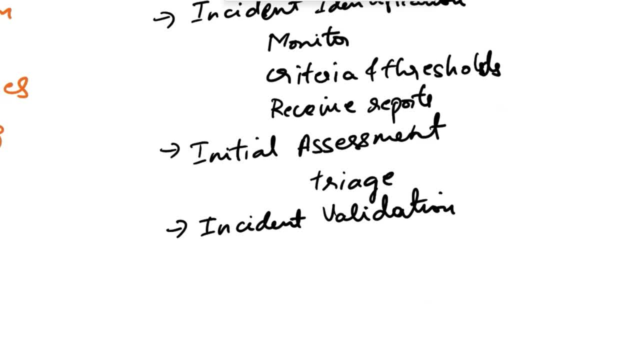 security incident or part of a broader attack campaign. And then we have data collection and analysis. Here we collect and preserve relevant data and evidence related to the incident, ensuring proper chain of custody and integrity, Then perform in-depth analysis of the collected data, logs, system artifacts or network captures. 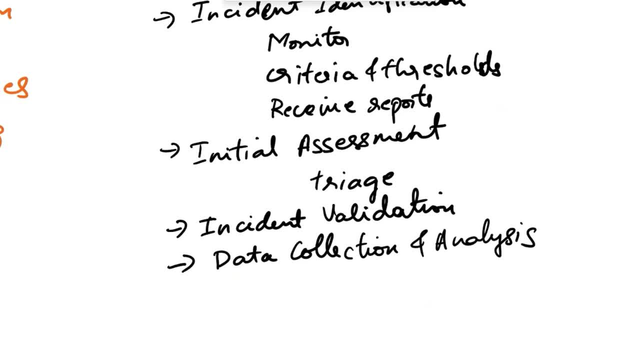 to understand the attack vectors, techniques and potential impact. Then we identify compromised systems, affected users or exposed data to assess the scope and severity of the incident. And then we use forensic techniques to reconstruct data and evidence related to the incident, ensuring proper chain of custody and integrity. 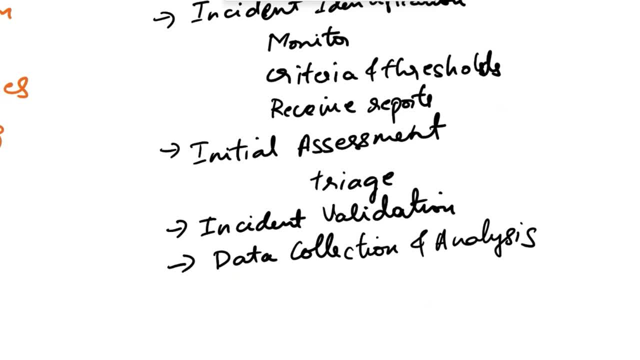 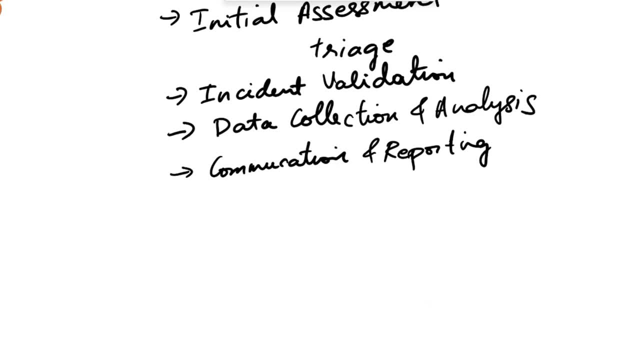 We also identify the timeline of events and identify the root cause of the incident. And then we have communication and reporting. This involves the communication with stakeholders, incident response team members and management to provide updates on the incident investigation and analysis. And then we document findings, observations and analysis results in incident. 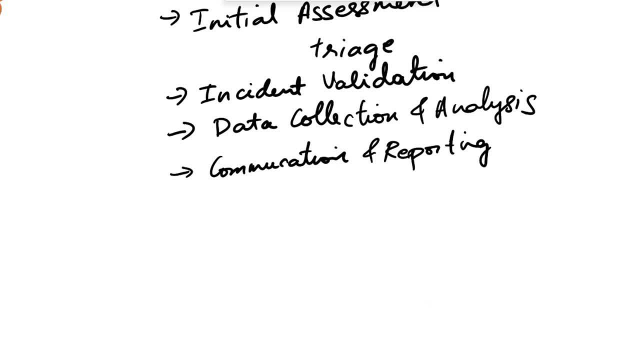 reports or case files, ensuring accurate and comprehensive documentation. Then we share the relevant information with external entities, such as law enforcement, vendors or other organizations, as necessary and based on organizational policies and legal requirements. So the detection and analysis phase is crucial for understanding the nature. 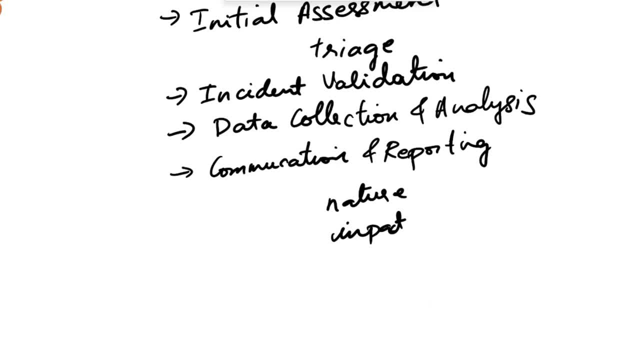 and impact of the incident. It involves a combination of technical analysis, forensic investigation and collaboration within the incident. So also we do the protection of the system, protection of the wszystkich for the treatment process and also the source of the custodial evidence. 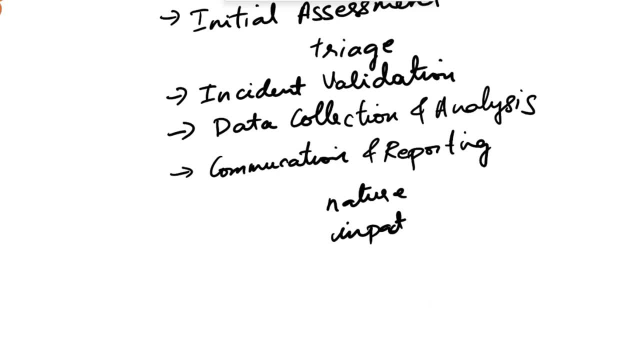 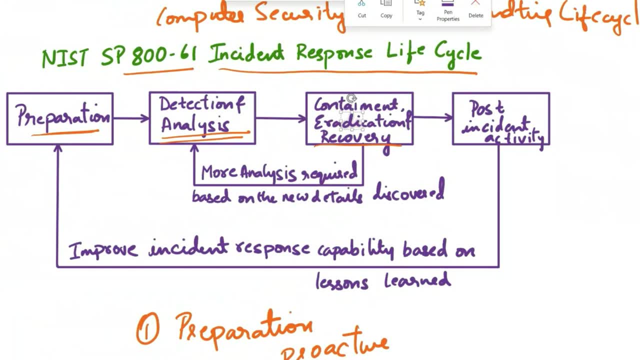 Formation of the mechanism也是 cycles by which one personal appropriator or the service provider can plan the route to the incident elements and also functionally evaluate the relationship with Popular Jagguers, internal and external organizations, and then carry out historical and futile investigation on services that 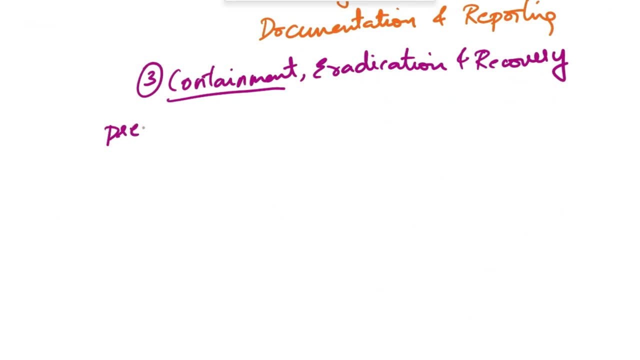 play a vital role in the treatment process. The next phase of finding the ultimate solution is containment, eradication and recovery, And this part is required for all of the factors mentioned. it again Once we know the proper funcion. allezant scouting applications. 루�ang genesis. 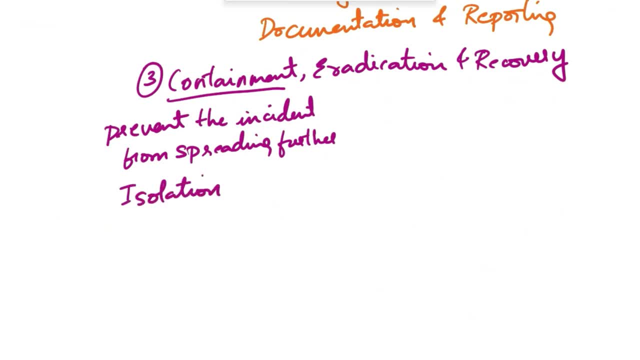 التandro- defensive tasks and response team needs to be prepared. Okay, now we know about preparation and detection and analysis. The next phase is containment, eradication and recovery. First, let's see about containment. The primary goal is to prevent the incident from. 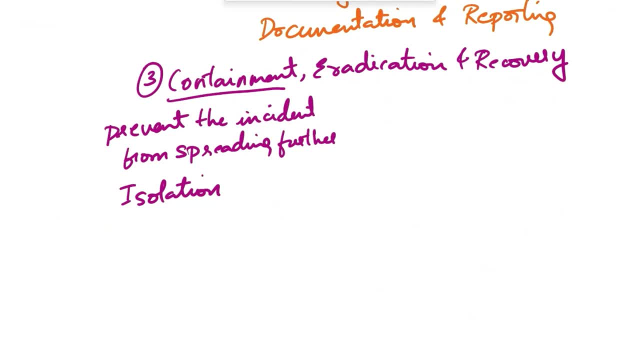 affected systems or network segments to minimize the impact and prevent the incident from spreading to other parts of the environment. This may involve disconnecting compromised systems from the network or segregating them into isolated segments. Then we have quarantine. Here we quarantine any suspicious files, network traffic or other artifacts associated with the incident. 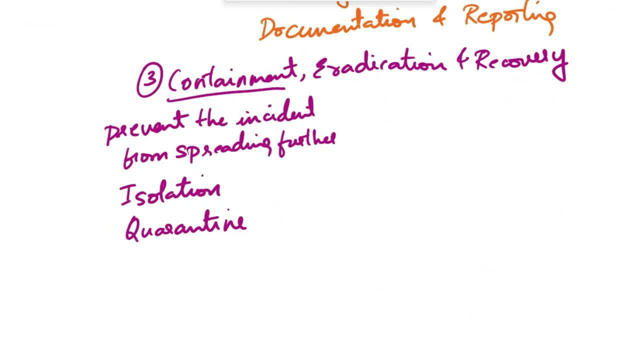 This helps prevent further propagation and allows for analysis and investigation. And then we implement temporary user access controls or restrictions to limit the privileges or actions of affected users. This helps prevent unauthorized access or malicious activities during the incident response process. And then is the communication. Here we establish effective. 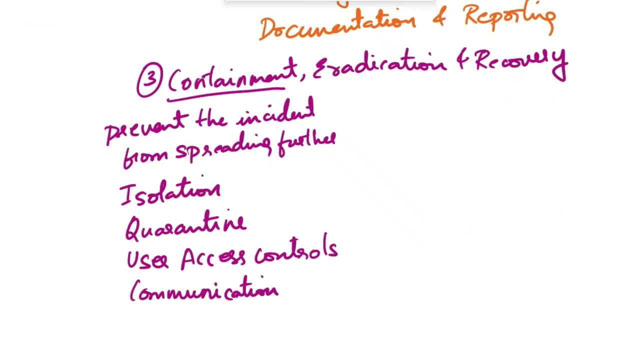 communication channels within the incident response team and with other systems. This helps prevent further propagation and allows for analysis and investigation Stakeholders to coordinate containment efforts. This includes notifying relevant personnel about the incident and providing instructions on appropriate actions to take. The next one is the 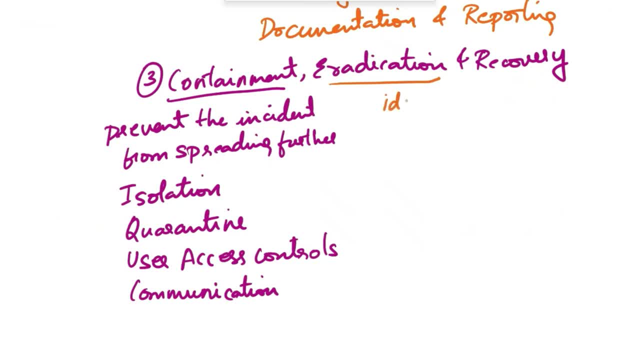 eradication phase. This focuses on identifying and removing the root cause of the incident. The main objective is to eliminate the vulnerabilities or malicious presence that allowed the incident to occur. Some of the steps that are typically involved in the eradication phase- Our first one is investigation. Here we conduct a thorough investigation to identify the root cause. 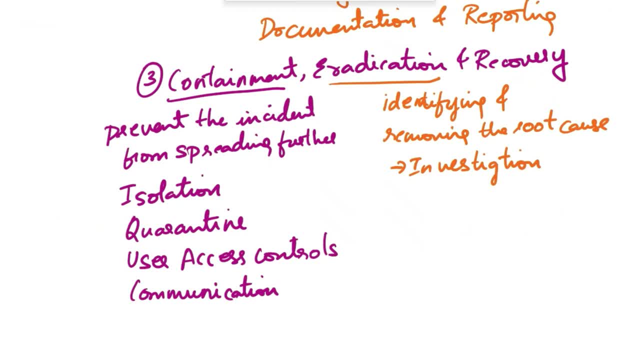 of the incident. We analyze logs, system snapshots, network traffic and any other relevant evidence to understand how the incident occurred and what vulnerabilities were exploited. Then we have patching and remediation. Here we apply necessary patches, updates or configure changes to address. 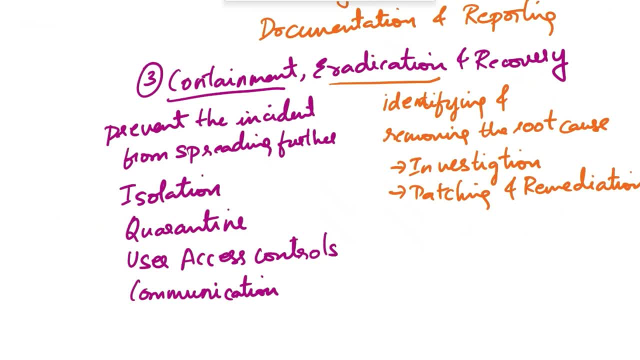 the vulnerabilities that were exploited. This may involve updating the system or configuring the software, firmware or hardware components, or reconfiguring systems to align with best security practices. And then we have malware removal, That is, to remove any malicious software or code that was discovered during the incident. Here we use appropriate tools and techniques to detect and 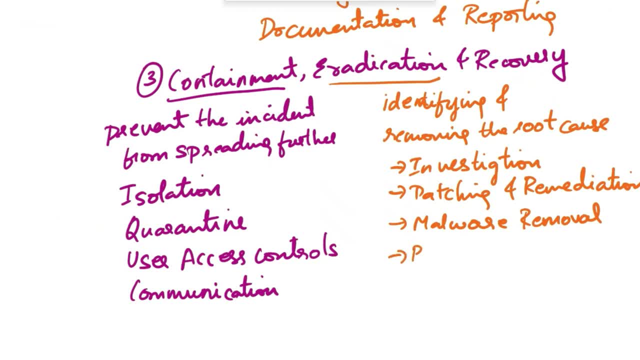 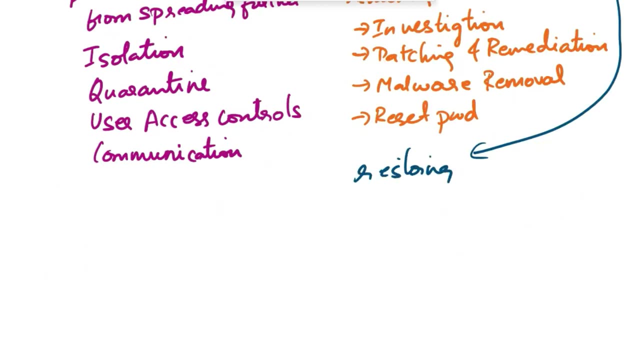 eliminate malware from affected systems, And then we reset passwords for compromised accounts or systems to prevent unauthorized access or further exploitation. In the next one is the recovery phase. The recovery phase involves restoring the affected systems and services to a known good state. The objective is to bring back operations to normal and ensure the 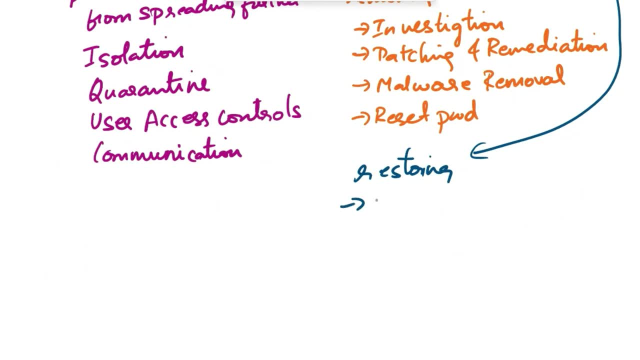 integrity of the environment. This involves steps like system restoration, that is, to restore affected systems, applications and services from trusted backups or rebuild them as necessary, Also to ensure that the restored systems and services are in good state. So here we have patching and 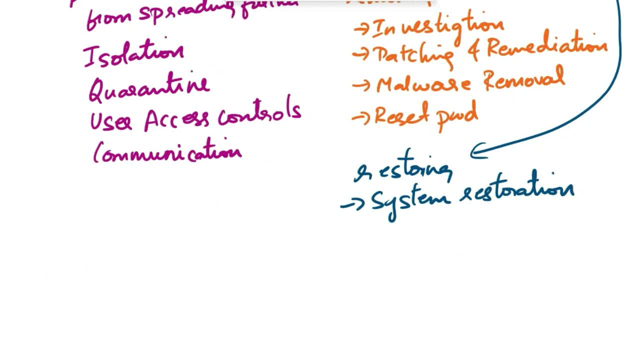 components are free from any compromise and thoroughly validated before reintroducing them into the production system. Then we have verification and testing. Here we verify the integrity and functionality of restored systems through rigorous testing and validation. We conduct vulnerability assessments, or pen tests, to identify any residual vulnerabilities, and then we 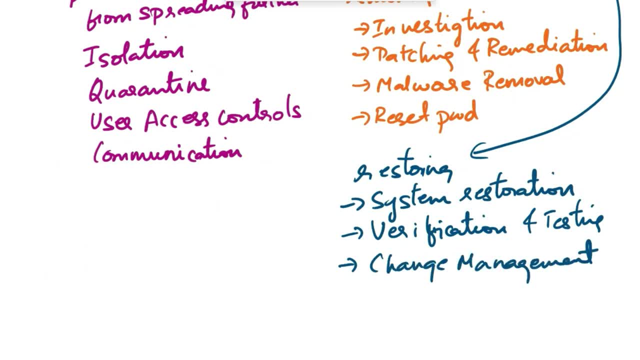 implement appropriate change management processes to track and document any changes made during the recovery phase. This ensures proper configuration management and facilitates further audits or investigations. So, to summarize, the containment, eradication and recovery phase requires a systematic approach to minimize the impact of the incident, remove the root cause and restore 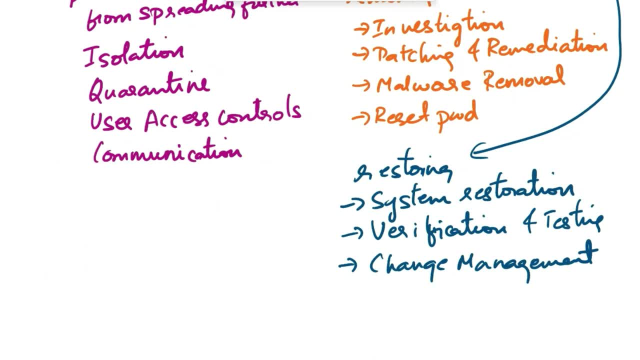 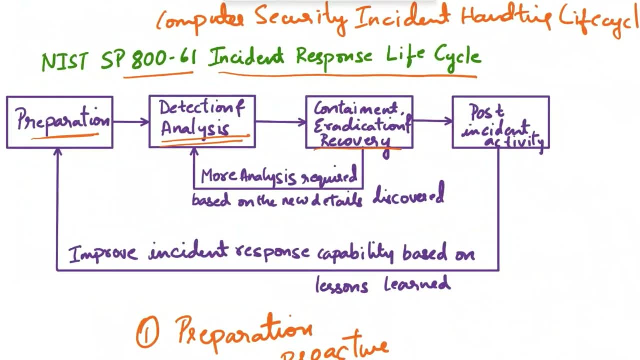 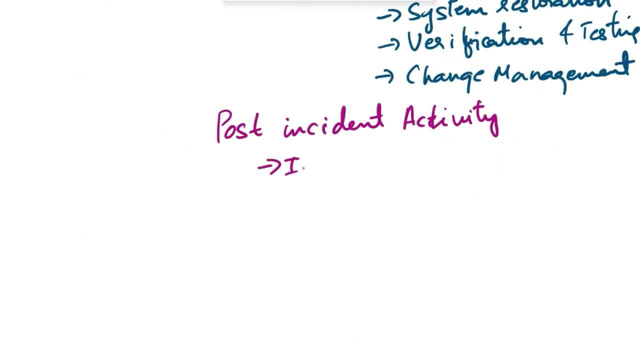 the affected system to a secure and operational state. Okay, Now we have discussed the first three phases: preparation, detection and analysis, containment, eradication and recovery. The final phase is the post incident activity. This phase involves incident documentation. Documenting the details of the incident is essential for 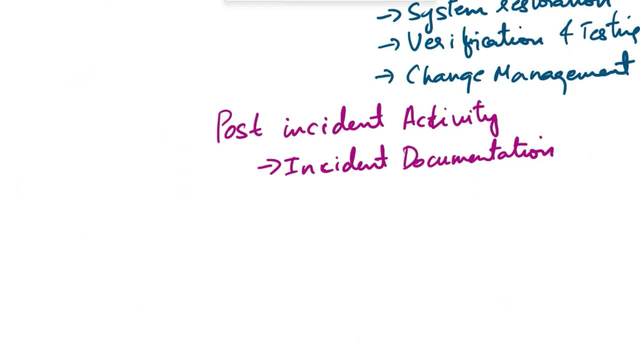 future references, analysis and learning. This includes capturing information such as the incident timeline, actions taken, evidence collected and outcomes. Thorough documentation ensures that a comprehensive record of the incident is maintained. Next, we have evidence preservation. Here we preserve any evidence related to the incident. 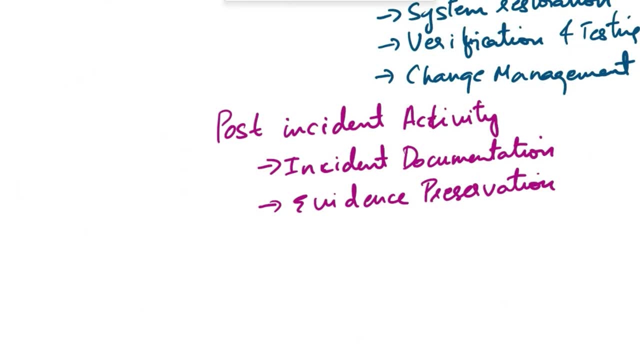 for potential legal, regulatory or internal investigation purposes. This involves securely storing logs, network captures, system snapshots and any other artifacts that might be relevant for future analysis or legal proceedings. And then we have post incident review. Here we conduct a post incident review or lessons learned session to evaluate the effectiveness of the 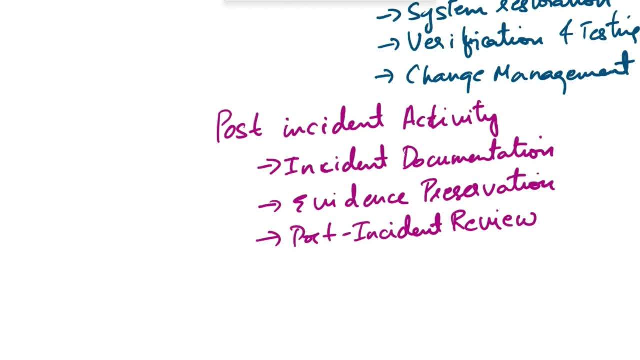 incident response process. This review involves analyzing the incident handling approach, identifying areas for improvement and documenting recommendations for enhancing future incident response capabilities. Then we have reporting. Here we prepare incident reports summarizing the incident, the response actions taken and any recommendations for mitigating similar incidents in the future. These reports are typically shared with. 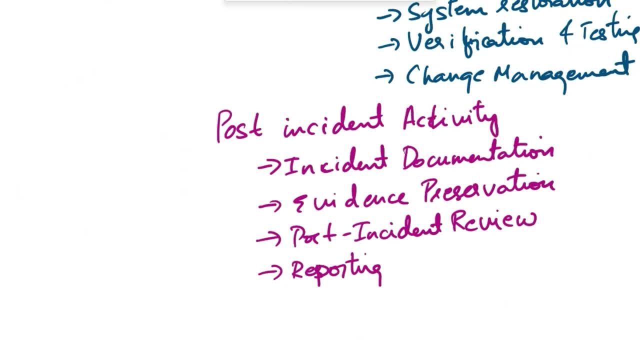 management, stakeholders, legal teams and other relevant parties, as required by organizational policies and legal obligations. Then we have communication and notifications. Here we share appropriate information about the incident with stakeholders such as management, customers, partners or regulatory bodies, as necessary. Transparent communication helps maintain trust. 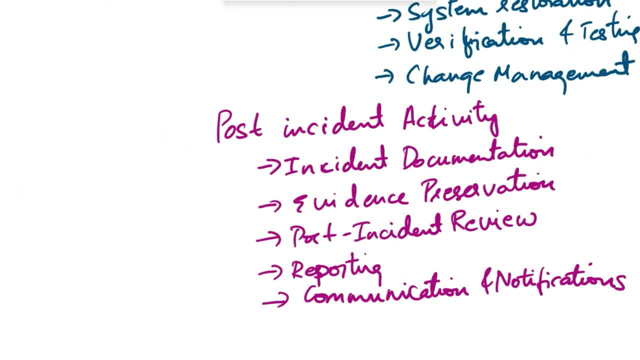 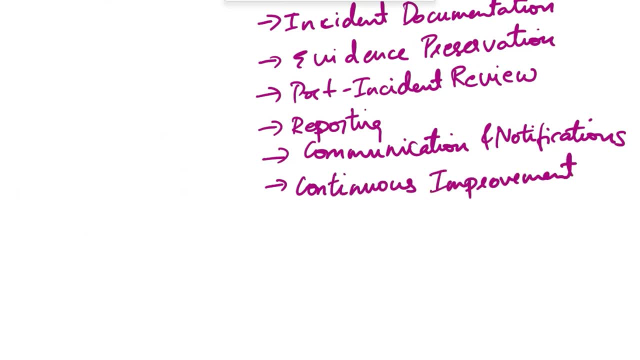 and facilitates collaboration in mitigating future risks. And then is continuous improvement. Here we use the insights gained from the incident response process to improve security measures, policies, procedures and incident response plans, And then update the incident response policy plan and related documentation based on the lessons learned to enhance future incident 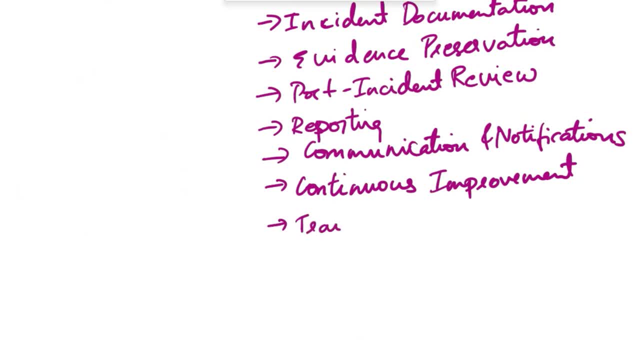 handling capabilities. Then is training and awareness. We identify any training, training or awareness needs that arose during the incident response process. This may involve providing additional training to incident response team members, users or employees to improve their security knowledge, incident detection or response skills. 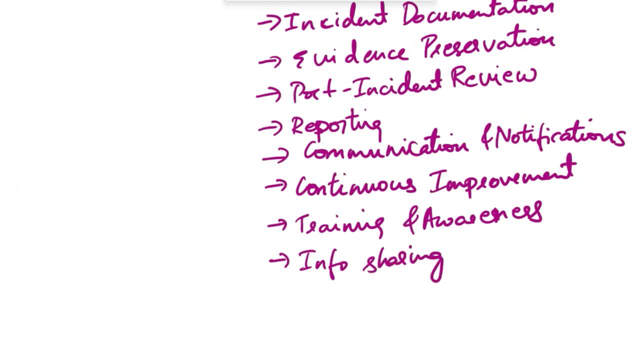 Then there is information sharing. We share relevant information about the incident with external entities such as the other organizations, industry forums or information sharing communities contributing to collective security efforts. Sharing incident details and insights helps others enhance their security posture and prevent similar incidents. So the post incident phase emphasizes. 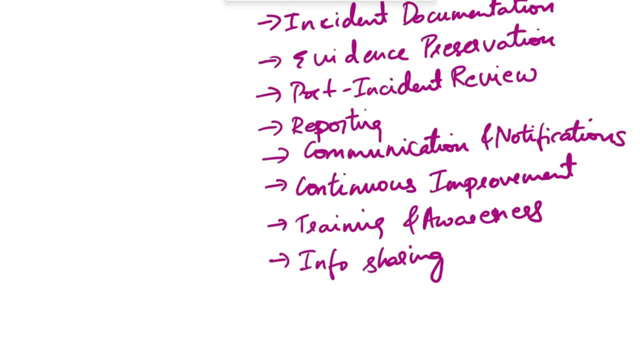 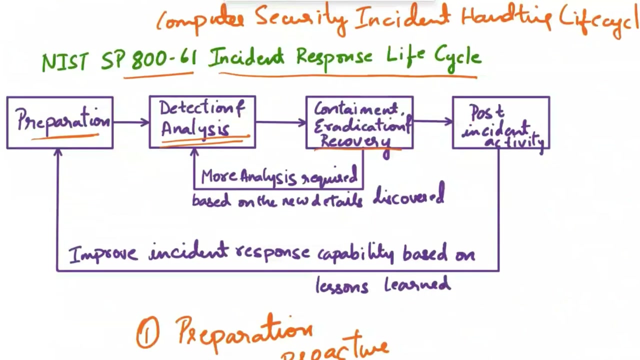 the importance of learning from the incident and using that knowledge to strengthen security practices and incident response capabilities. By conducting a thorough review, documenting lessons learned and implementing recommended improvements, organizations can enhance their resilience against future incidents. Okay, now we know all the four phases of the incident response life cycle. 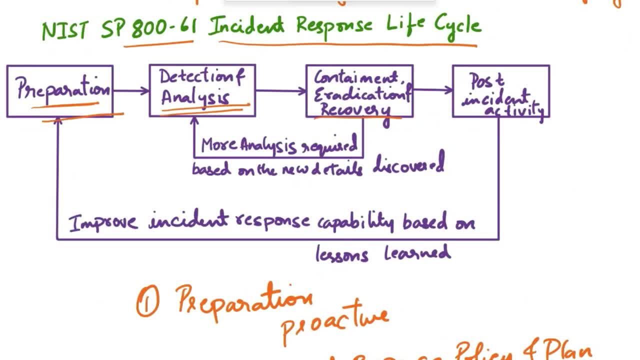 So first one is prepare, where you establish incident response policies, plans and teams and define roles and responsibilities and set up security controls. Then we have detection and analysis phase, where we monitor systems for indicators of compromise, validate security incidents and analyze data to determine the scope and impact of the incident. 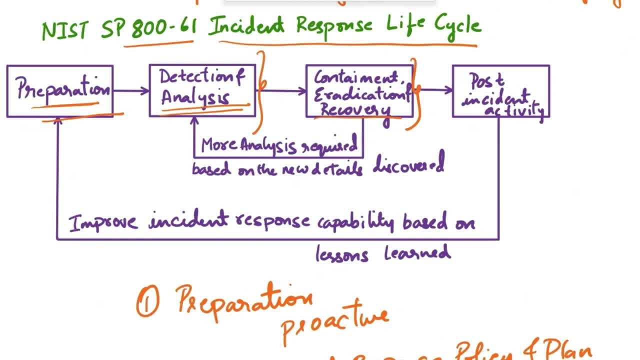 Then we have containment, eradication and recovery phase. Here we contain the incident, remove the root cause, restore affected systems and prevent further damage or compromise. And whenever here in the third phase we require more analysis, we go back to the second phase.